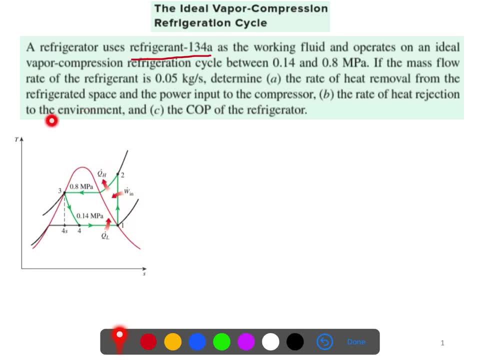 We need to calculate the rate of heat rejections to the environment. We need to calculate that means Q, H and finally C of E. So we will start with the you know calculations. So at first we we should write down some assumptions. So, as you know, we will write down some similar. 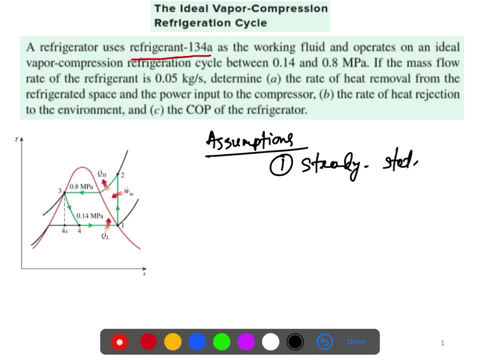 assumptions. We will say this is a steady state device and finally, we will say that the kinetic and the potential energy change it will be. let us say we can write it down like this: So it will be equivalent to 0. It is negligible. So that is all of our assumptions. 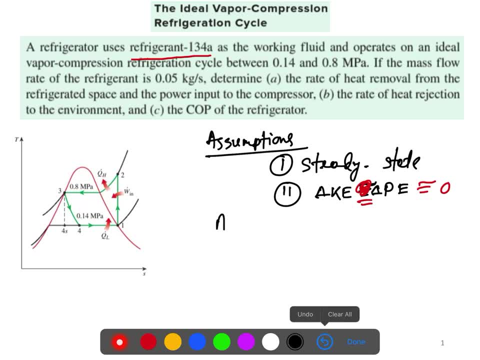 So now, when we will start with the analysis, So foriferation analysis, actually try to understand this T 있고요 diagram. This is the phase 1,, 2,, three, four. okay, So four different phases here to different states. You can see this is as interest compression. 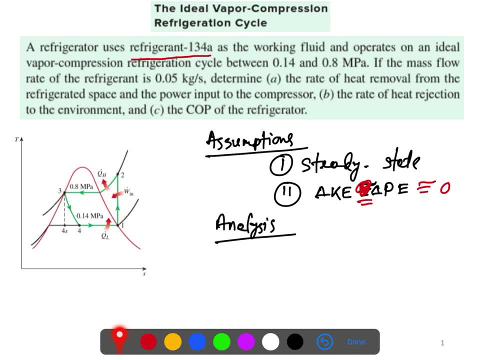 happening in this section We used situation for ideal vapor compression cycle in a small, if you can remember, we discussed we use the expansions valve. due to the expansion valves, this point actually, if we use the turbine then it should be isentropic expansion here, then the point will be forest. but we use the throttling valve so it moves like here. so you, 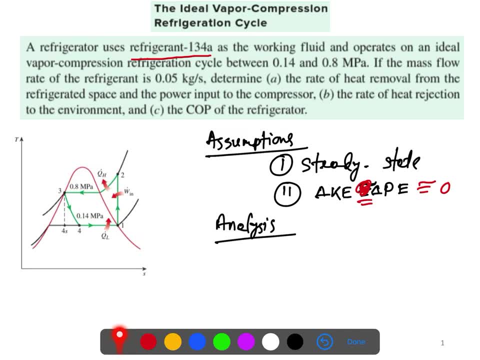 can say there's two points. it's. the difference is negligible. maybe that we will decide later on here. what you can see at this stage is saturated vapor state 2. this is superheated vapor and this is saturated liquid. right, this is the mixture reason. you know this from first up. you know first. 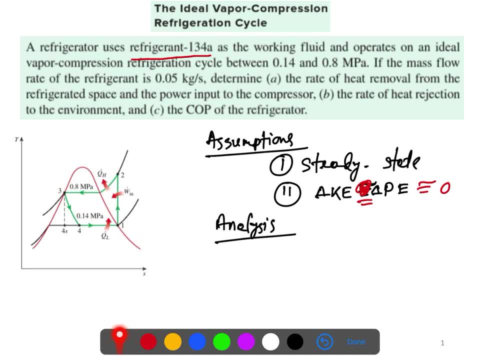 two, three weeks. we discussed this. so actually here, when we will start with analysis, the first thing we will do is we'll calculate the enthalpy's, because we're looking for Q, L, Q, Hayes and we said the kinetic and the potential energy is zero if I say, let's say that the heat theta equal, let's say m kinetic energy. you know, 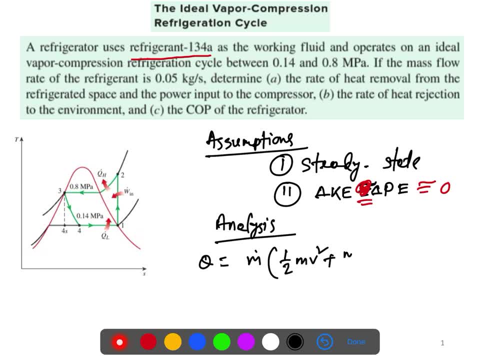 half m V a square. you know, mg Hayes, and you know we should not write mg Hayes. we can say when we put the mass, okay, I think let's say kinetic energy. I should write this a kinetic energy, potential energy and enthalpy. okay. so the kinetic energy, potential energy. 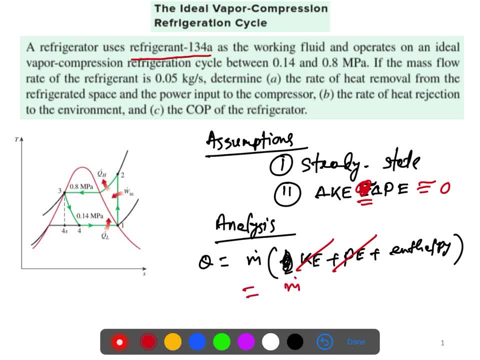 wall zero. so that means we need the mass into enthalpy, that means the enthalpy difference. if, if you can remember, if we want to calculate this Q L between this process one and four, so the Q L we can write, it is, you know, the, according to the formula we can. 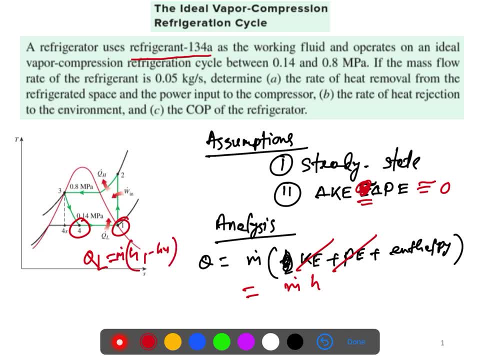 say Hayes one minus Hayes four, and as we have the mass flow rate, we need to include the mass flow rate here. so that means if we want to calculate Q, L, w a and Q Hayes, whatever it is, we need the enthalpy. so what I will do is, initially I will calculate the enthalpy for all of these four. 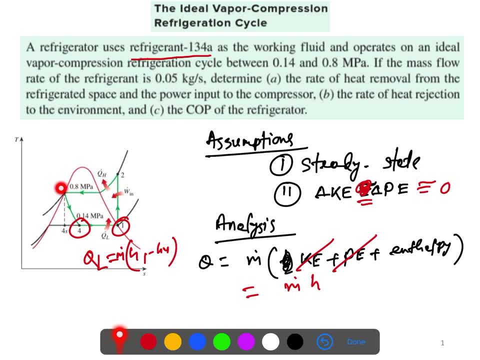 states one, two, three, four. so let's do that. if we want to do that, let's if we try to calculate the enthalpy for state 1, so for a state 1 we know the pressure. it is given 0.14 MPa, in the question you can. 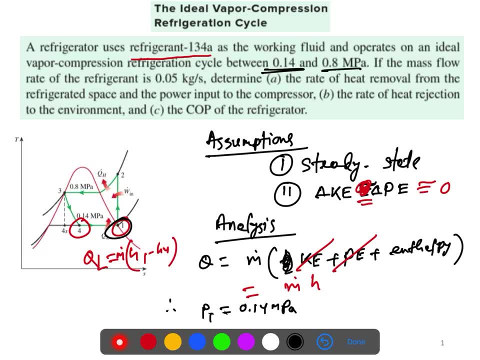 see the cycle between point 1 for 2.8. okay, so this is the pressure given. so for this pressure, we will try to understand- actually we'll try to get the enthalpy- and we will also calculate the entropy here. this is TS diagram we. 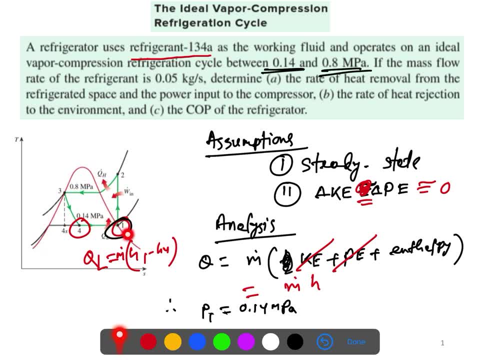 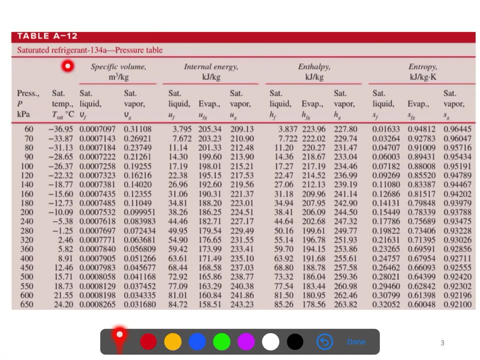 can easily do that. so this is the UDZ, you know, saturated saturation region. you see it is on the saturation type line. so we need to use actually table 812 here, the saturated refrigerant. you can see table 812. the pressure was 0.14 MPa. we can approximate this is you know how to. 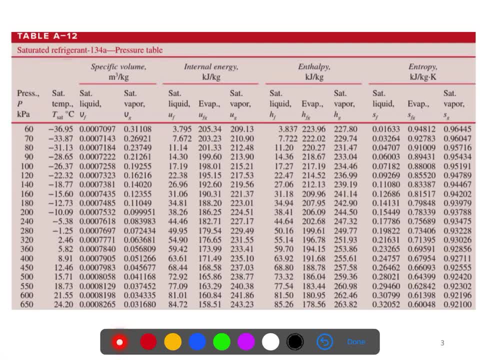 calculate actually this properties. so 0.140. so this is 140. so that means point it is kPa. so if we convert it into MPa it should be 0.14. so you need the enthalpy if we draw a line like this. you see, 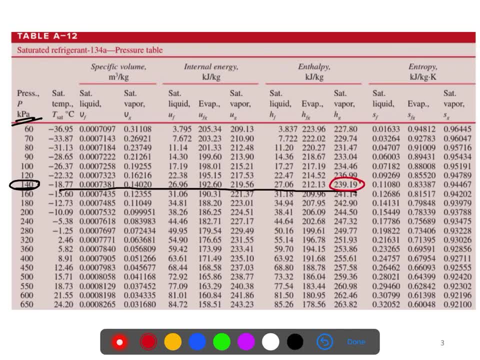 this is actually the enthalpy 239 point 0.19, and if you integrate the entropy, entropy is for the saturated region. you know it is 9, 4, 4, 6, 7. so this is actually the entropy and the enthalpy. I believe you know actually how to create these. 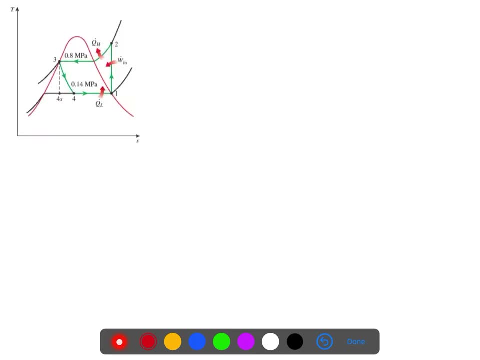 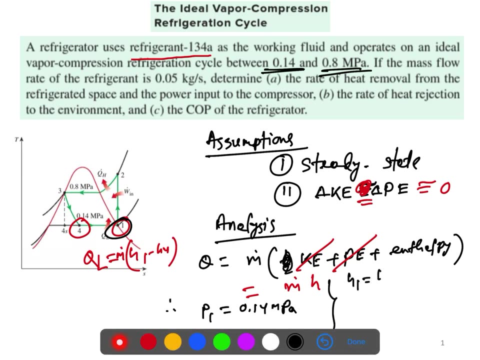 fellows. so now we will write down these two fellows. so what are you going to write down? so what? we can write down this two values. so what do you can write down? this right here is: we can say that H1. we can say it is equal to Hg at rate of 0.14 MPa. So 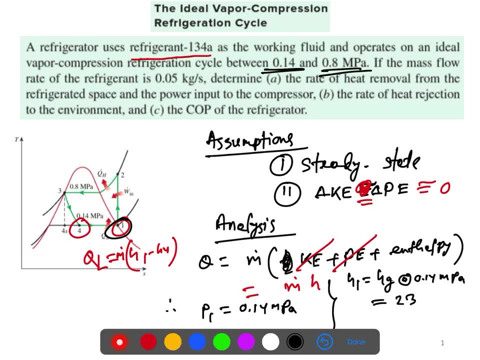 at this condition we can approximate. it is saturated, So 239.19 kilo joule per kg, and similarly S1, it will be 0.94467 kilo joule per kg Kelvin. So this is for state 1. So 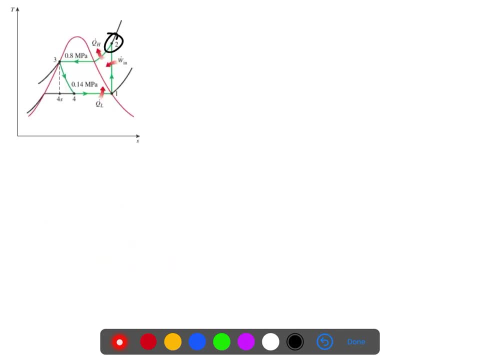 now if we go for this state 2.. So for state 2, what is the pressure? Pressure is 0.8 MPa and it is isentropic compression. So the pressure, you know the entropy, is S1 and S2, it is same. So it is isentropic change. So entropy is not changing. So it. 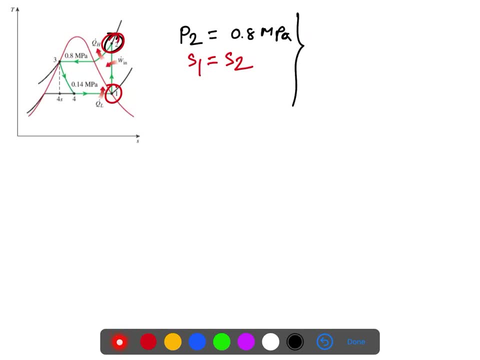 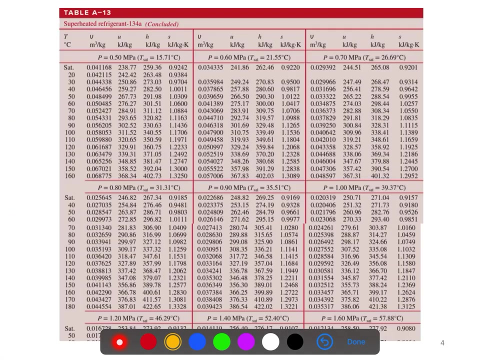 should be equal. So, at this state, at this state, we know the pressure, we know the entropy, and it is in the. in which region? It is in the superheated vapor region, right? So now what we need to do is we need to use the superheated. 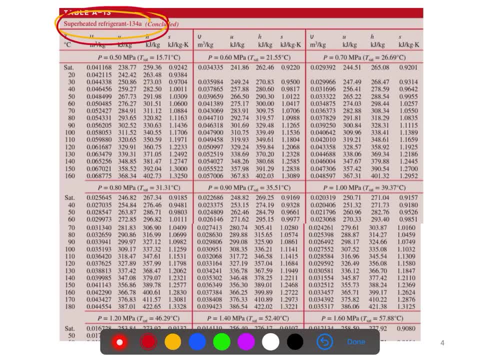 Refrigerant table. yeah here. So look carefully, the pressure is 0.8. so that is the point. and we have got the entropy is, you know, 0.94467.. So look where it is 94467.. So you will you. 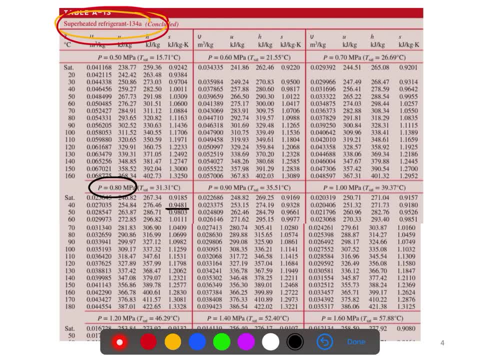 will see entropies. this is nine, four, eight one, right, so this is nine on eight one. so you need to- and this is actually the corresponding enthalpy- so you need to do some interpolations. so you know how to do this interpolation, so i'm not going to show you. i'll write down the final value. the haste to it is: 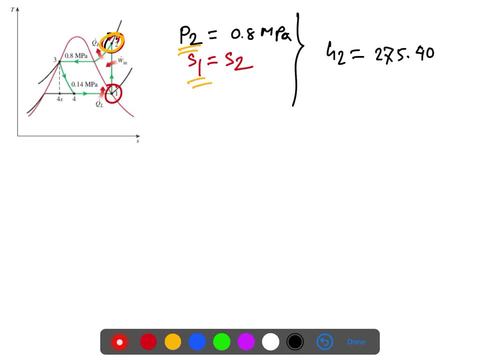 equal to 75.40 kilojoule per kg. so that's it now for a state three. you know p3, so state three: this is same pressure, 0.8 mpa. so for this pressure we can write down: okay, the haste to it is equal. 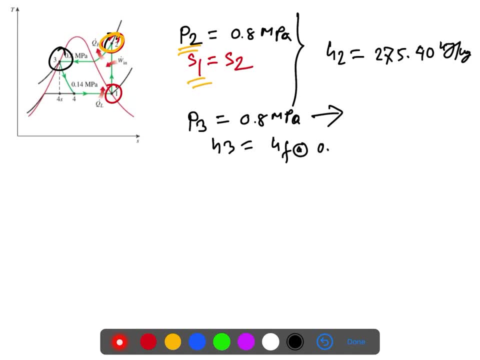 hey, say, at the rate of, you know, 0.8 mpa, because it is on the saturation in the situation. so this is the pressure, 0.8 mpa. so this is the pressure, 0.8 mpa. so this is the line. so this is in a saturated liquid, so we will get it from the table. I'm not 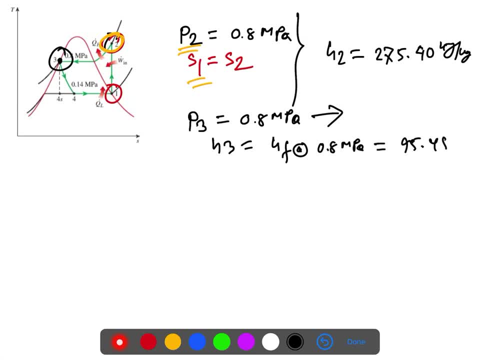 showing you again. so it is nine, five point four, eight kilojoules per kg, and we discussed earlier. this has three and has four. actually this is in between these two processes. we have a throttling valves. so since throttling process is isentropic and for ideal gas actually, enthalpy is function of T, right. so 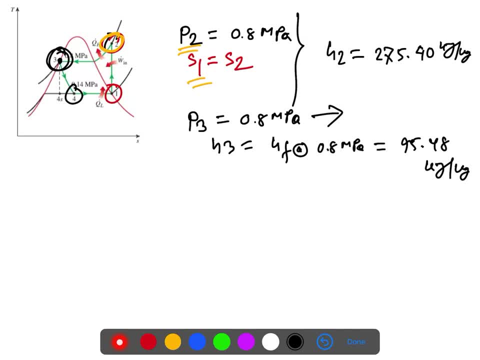 enthalpy is function of T, so T does not change for ideal gas during the throttling processes. here we usually replaced for. for ideal vapor compression, we replace the, you know the turbine and we use the throttling processes. so then this point moves to here. otherwise if it is turbine it should be in force. so 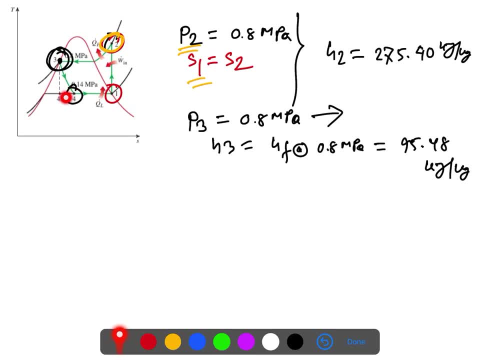 we assume that this change is negligible. okay, just for the simplicity, otherwise it will be complicated to solve this question analytically. so we said: this has three, the enthalpy, and has three and for has four they are. during the throttling process we said: there, you know, the change is negligible. 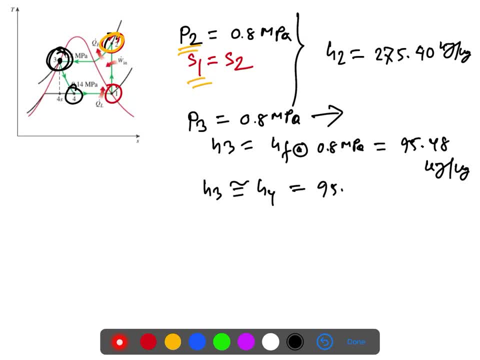 so we can say h3, h4. it is equal the same 95.48 kilojoule per kg. so we have got all these values. so now um see, the first part of the question is it was asking about the rate of heat removal from. 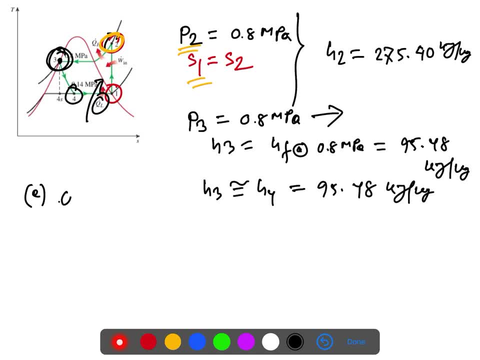 the refrigerant space. that means what is the ql? so if we want to calculate the ql, we know the mass flow rate, m and the enthalpy difference. so it is h1 minus h4, isn't it? so mass flow rate is 0.5. 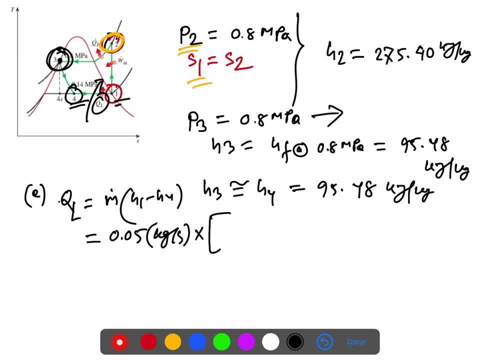 it is kg per second into h1 is, you know, 239.19 and it is 95.48 kilojoule per kg. so we will get ql. it is equal 7.19 kilowatt. so this is um. actually, you know the amount of heat removal from the refrigerant space. 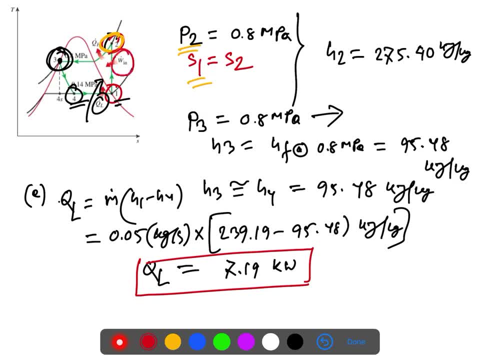 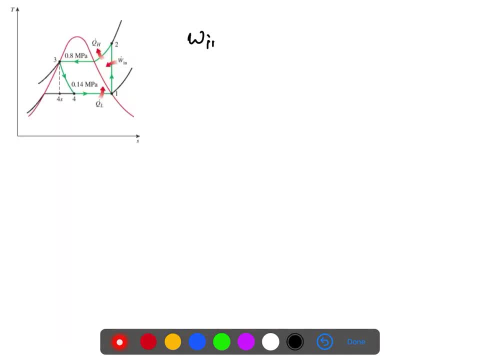 so the second part is asking about the work input, how much work we need. so if we actually calculate the work input, let's say the work in, so that means this one. so there's the enthalpy difference between the one and two. so we can say it's mass flow h2 minus h1. right, this is simple formula, you know. 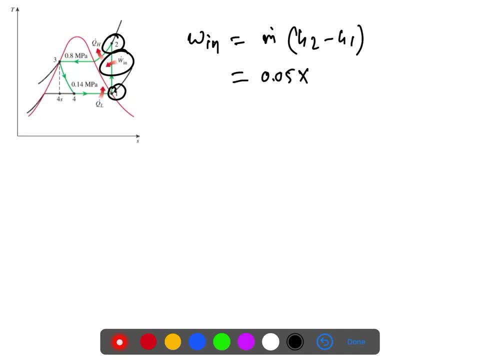 so the muscular rate: 0.0 5. i'm not writing the units again and again. so h2 is um, you know calculate it so it will be 1.81 kilowatt. so this is actually the work in. so we have got the work in. we have got the heat removal from the refrigerator into space. now the third part of this question it is asking about, you know, the rate of heat rejections from the coolant. 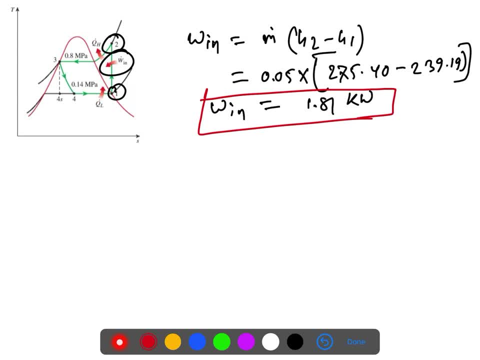 the environment, um, you know, to the environment. okay, so that means q hays. we need to calculate the q is how much it where the system is rejecting to the environment. so q hays, um, it is again same. we can say m and it will be from this process, two and three, so you can say it is h2 minus h3. 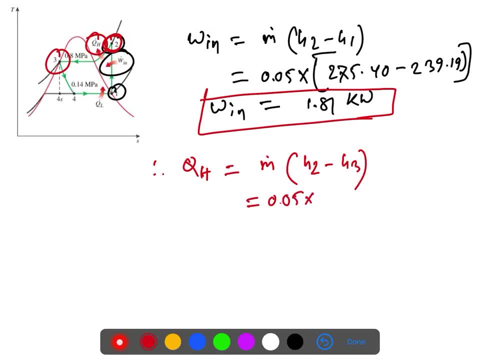 so m is 0.05 and h2 is, you know, 275.40, h3 is um, we calculated h3 is 95.48. so this value, it will be q hays, you know it will be nine kilowatt. so this is, you know, the q hays. so in other words, we can. 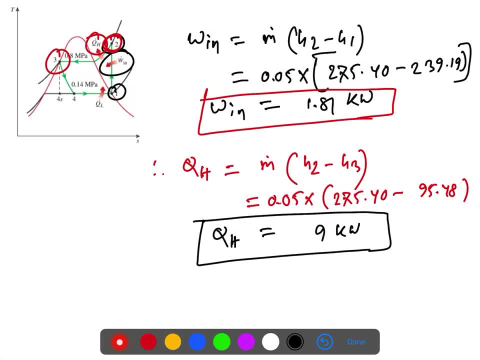 we can. we can calculate this q hays- um in other way. there is the formula: actually q hays, it is q l over q. sorry, it will be the the work input. so if you um use this formula, even you will get q hays, okay, so that's the same thing. 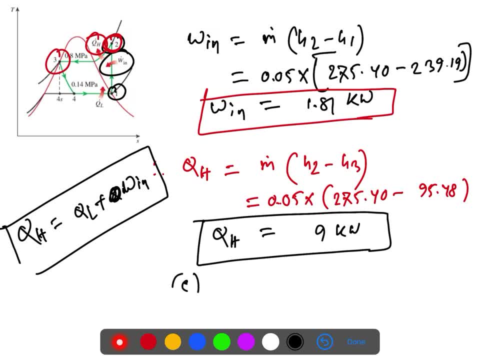 so now what we will do is the last part of this problem is we need to calculate the cop, the coefficient of performance, cop of the refrigerator. so cop of the refrigerator, it is actually called, you know, the the amount of heat removal from the refrigerant space. that means that's actually the desired output and the working. so we discussed- all of you know this- 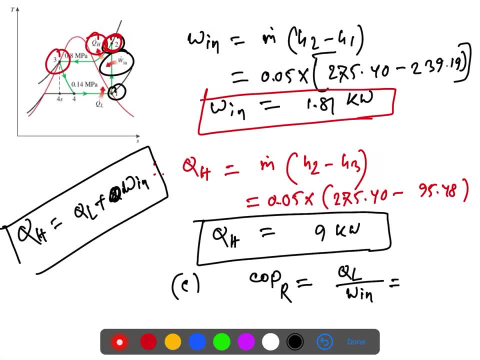 formula we discussed in a couple of weeks back. we discussed uh during the lecture as well- um, so it is ql over the lean, so ql is 7.19. it is kilowatt de blin is 1.8 on kilowatt, so it is 3.97. it's a dimensionless. 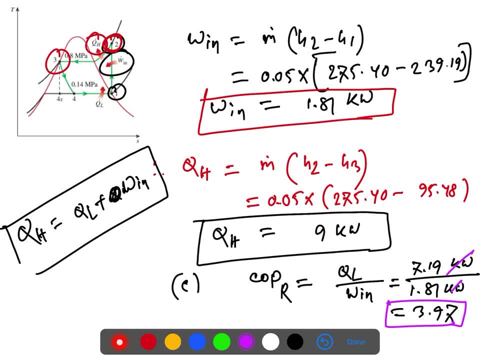 unit um, because we can simply eliminate this kilowatt here. so that means the refrigerant, this is the coefficient of performance of the refrigerator. so that means the refrigerator removes, um, you know, among four units of thermal energy from the refrigerant space for each unit of the electric.